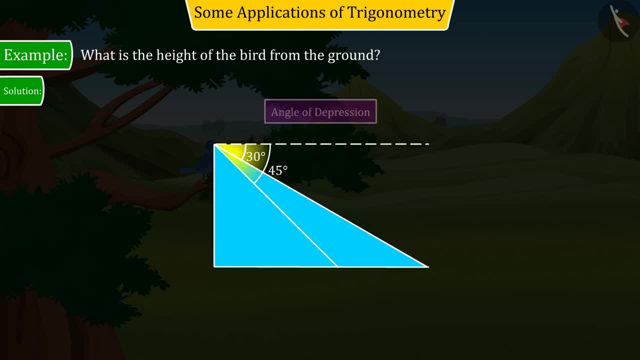 let us construct the figure, Let Mn be the height of the bird from the ground denoted by h, And let's represent the first position where the rat is seated by point P, In that case, the angle of depression made by the line of sight and the horizontal line of the bird sitting on. 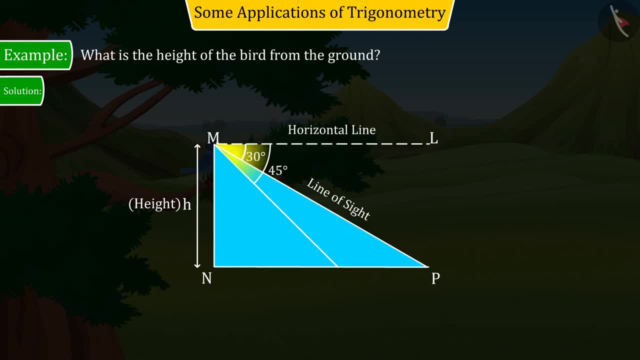 the branch is 30 degrees. Looking at the figure, we find that Pm is a transversal line of the angle of depression. Therefore the angle of depression is a parallel line of Lm and Pn. Therefore in this case we can say that angle Lmp and angle Mpn are alternate angles. So 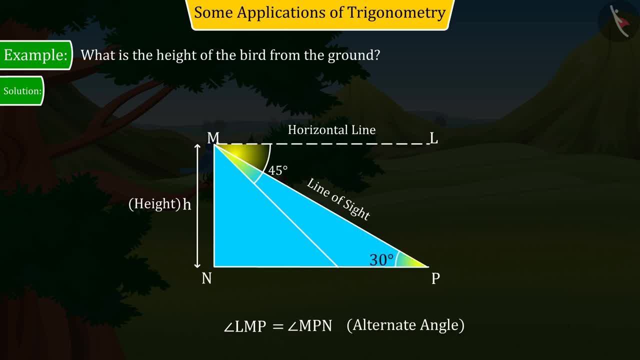 they will be equal. And in the second case, when the rat travels 20 meters towards the tree, the angle of depression becomes 45 degrees, assuming the distance from point O to N is x meters. Now let us figure out how the angle of depression formed by the line of sight and horizontal 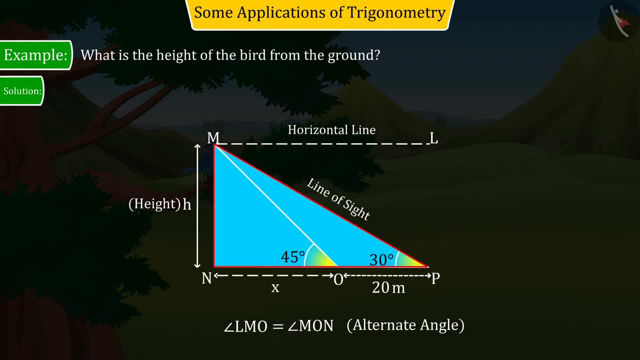 line is 45 degrees. Therefore, in both the above situations, the following figure is obtained, Since we have to find the height of the bird from the ground. So let's discuss triangle Mnp. In triangle Mnp we can see that the measure of sight Mn will be h and the measure 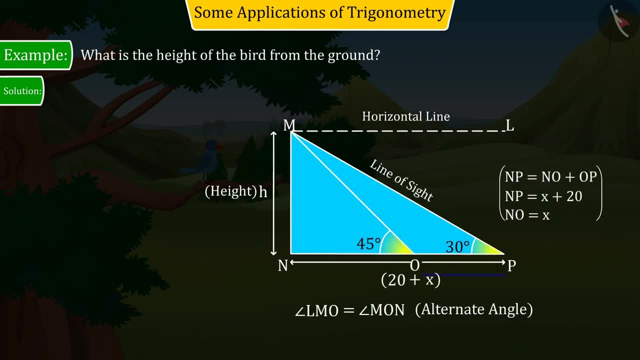 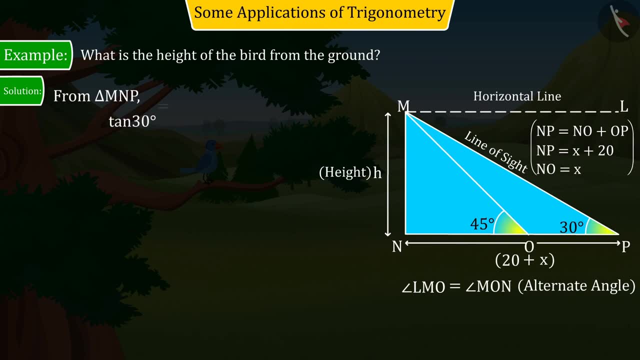 will be 20 plus x. So, with the help of the information obtained from right angle triangle, MNP and trigonometric ratios, the value of tan 30 degrees is obtained as MN by NP On substituting the values of sides MN and NP in tan 30 degrees and solving it. 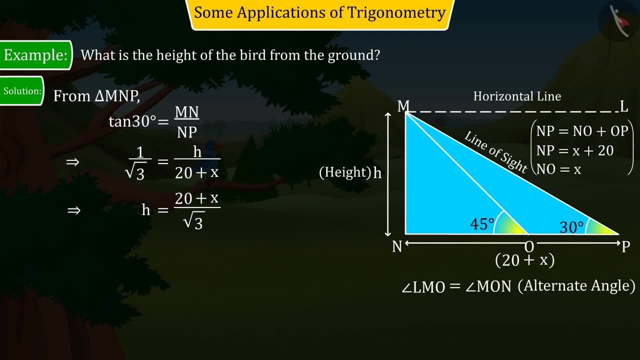 the value of h is obtained as 20 plus x by square root of 3, which is not a complete solution, because here the value of x is unknown. Let us represent it by equation 1.. Now let's talk about triangle MNO. With the help of trigonometric ratios we can see that: